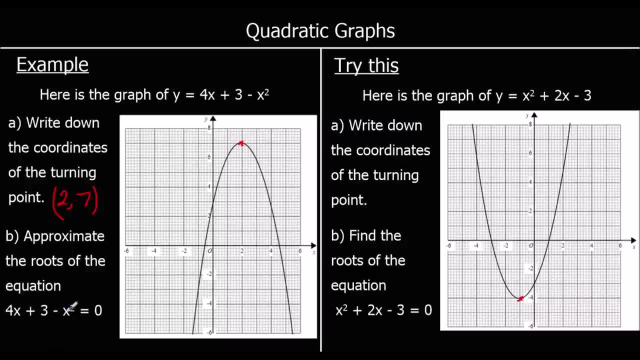 Approximate the roots to the equation: 4x plus 3 minus x squared equals zero. To find the roots of the equation we must start at negative y And we're going to approach the first and extreme. Let's go back to square root of x, So we've got equal. To word stainless and equal. We've got quitting of x on y, So we must find the roots and the ROB's method, which are 2,7, and zero, 1, and 1, plus pi, by both negative x squared. 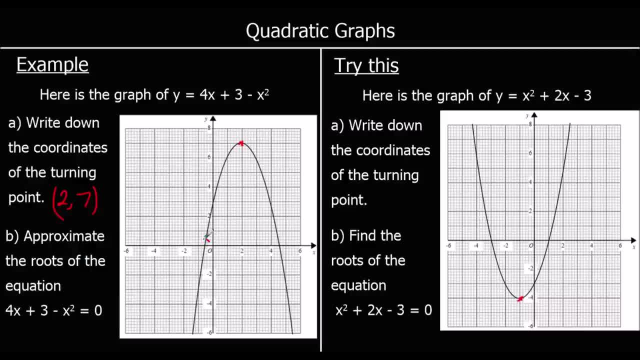 from an equation on a graph. we look at where it crosses the y-axis, so where y is equal to zero, so y has been switched for a zero. so y is equal to zero when it crosses the x-axis. so these two points are the roots and they are at 4.6. 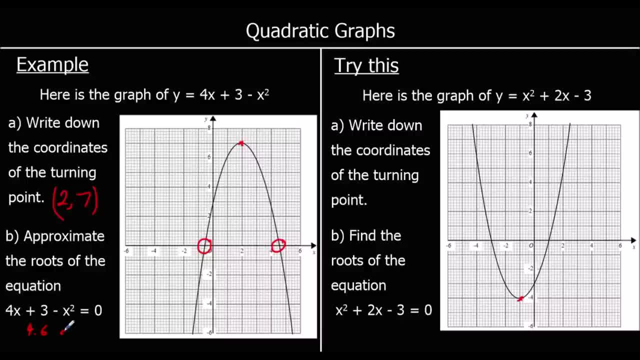 and so there's two solutions. it's a quadratic. we usually get two solutions and negative 0.6. okay, one for you to try. so pause the video and give it a go. so this time we've got the graph of y equals x squared plus 2x minus 3. 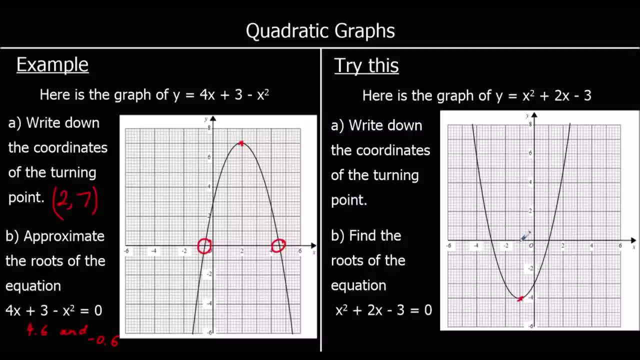 the coordinates of the turning point are at negative 1, negative 4 and the roots. so we're looking where it crosses the x-axis. so you see y has just been switched for a zero. so where y equals zero is where it crosses the x-axis. so we've got negative 3 and 1. 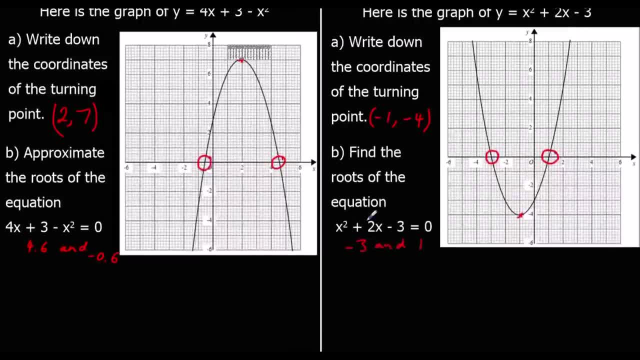 so in this example we could have also worked that out by factorizing, so we could have put it into brackets: what multiplies to make a negative 3 and adds to make a positive 2, so it's plus 3 and minus 1. so what makes the first bracket zero? that would be negative 3. 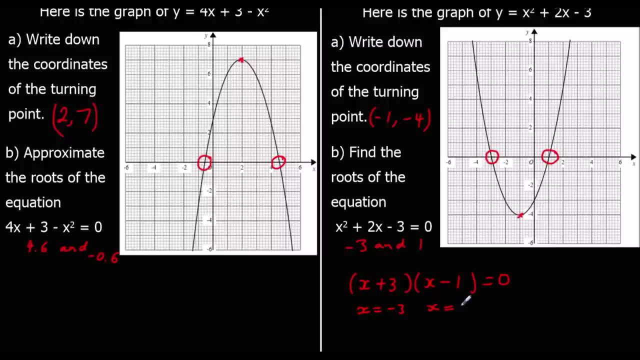 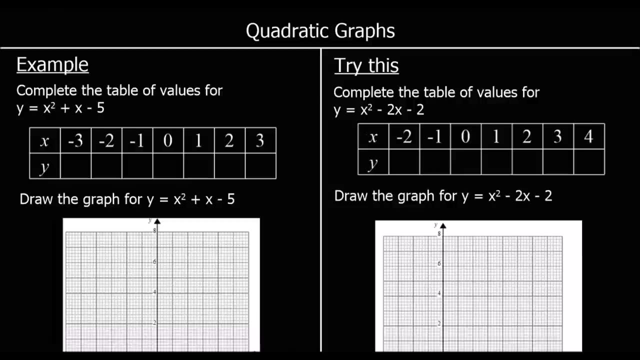 and what makes the second bracket zero? that's 1.6. and what makes the second bracket zero? that's 1.6, one positive one. so we could have solved it by factorizing, but we can also solve it by looking at the graph. here we're being asked to draw a quadratic graph. so the first step we're going. 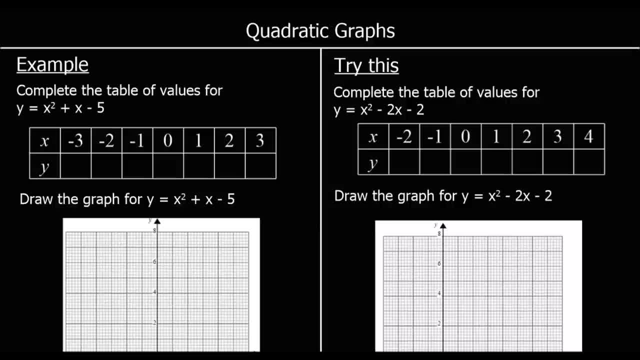 to complete the table of values and then we're going to use the coordinates that we work out to draw the graph. so you may have a calculator for this question. if you do have a calculator, you should use brackets to substitute the numbers in, so you should use brackets around the numbers. so, wherever you see, 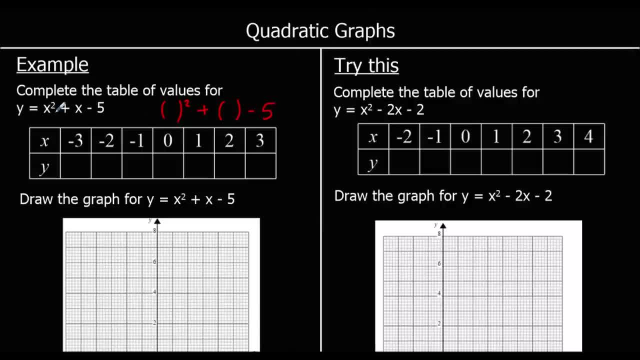 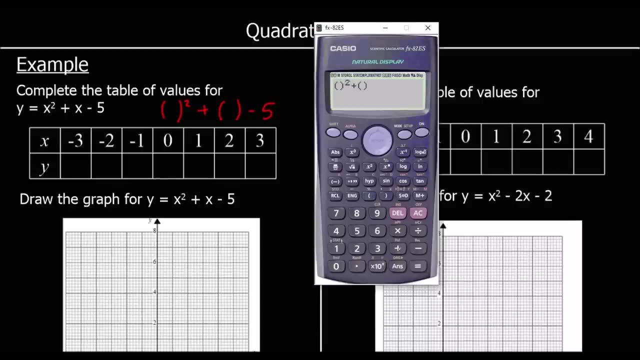 an x, replace it with brackets. so brackets squared plus brackets minus five, and then you can you put the x values into the brackets. so if you set it up like this and just switch the x numbers in the brackets, the reason we use brackets is because if you put a negative number in, 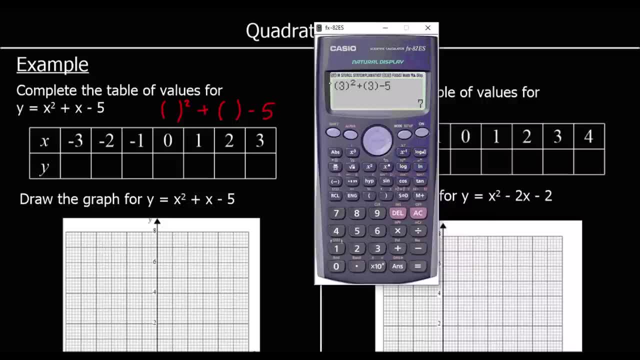 and the calculator and it's not in brackets, the calculator will not get the correct answer, so you need to put it in brackets so it knows you're doing negative 2 squared, not take away 2 squared. when x is 3, we've got 7. 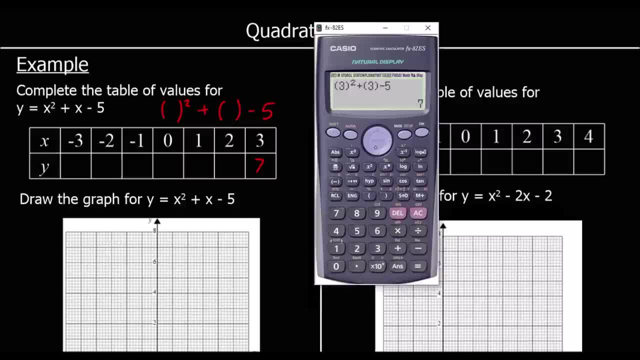 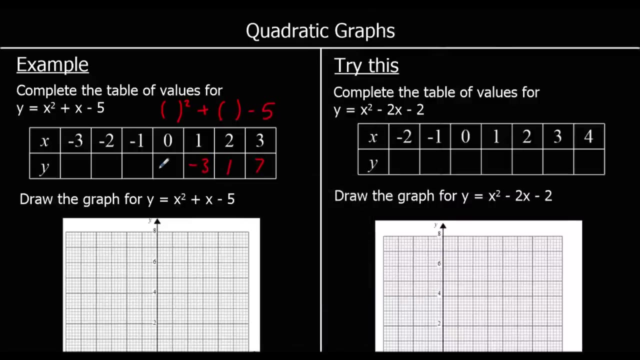 and we can change the 3 to a 2, and so when x is 2, we've got 1, when x is 1, we've got negative 3, when x is 0, we'll be negative 5, and you could probably see a pattern starting to emerge. 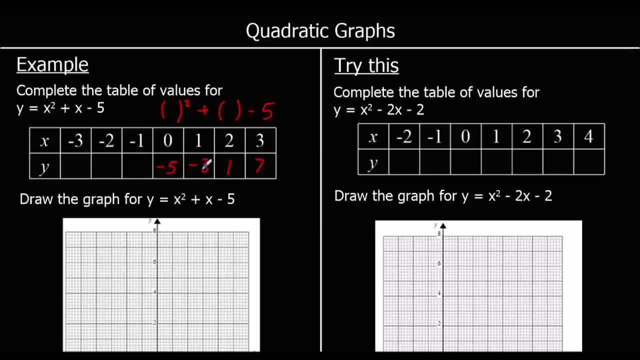 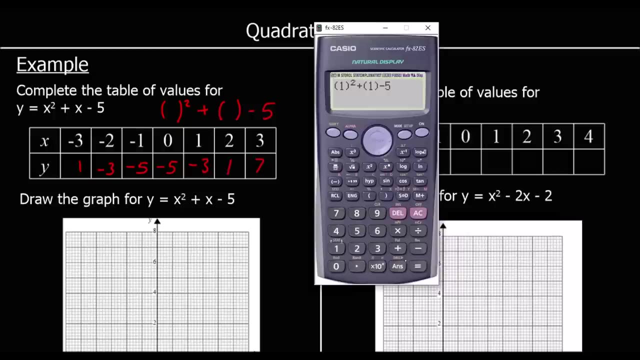 so it's gone down 6, down 4, down 2. the next one will go down 0 and then up 2 and then up 4, but you can check these on the calculator. so for negative 1 we've got negative 5, for negative 3: 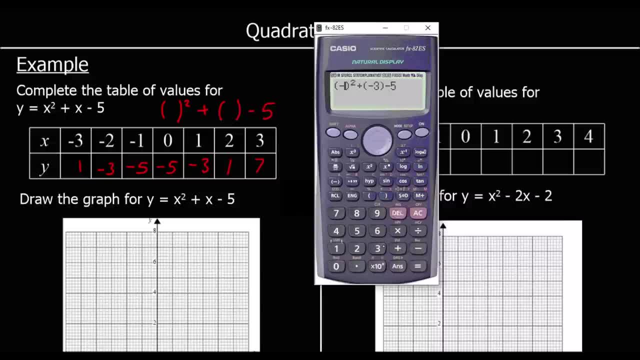 we've got 1, and let me just show you why. you're using brackets on the calculator. so if you just typed in negative 3 squared plus negative 3 minus 5, the calculator gets negative 17. so it is completely, completely got the squaring of negative 3 wrong. 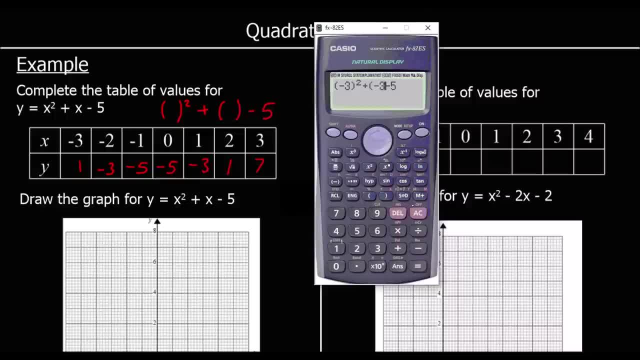 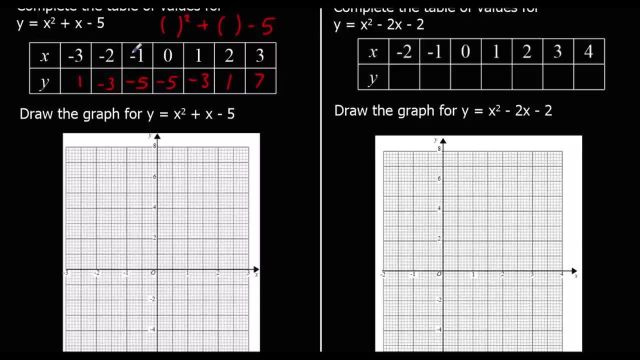 because it thinks you mean take away 3 squared. so use brackets when you're substituting into the calculator and we can plot these coordinates now. so each one of these is a set of coordinates. we've got negative 3: 1. negative 3: 1. 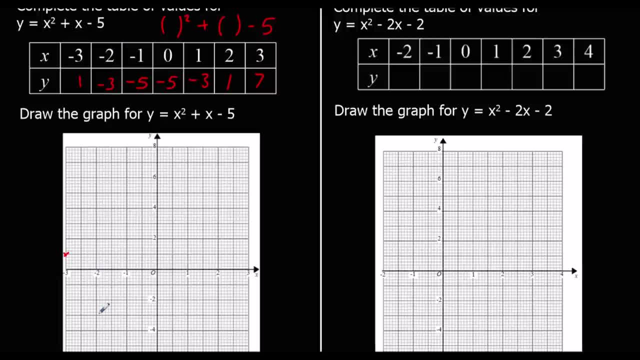 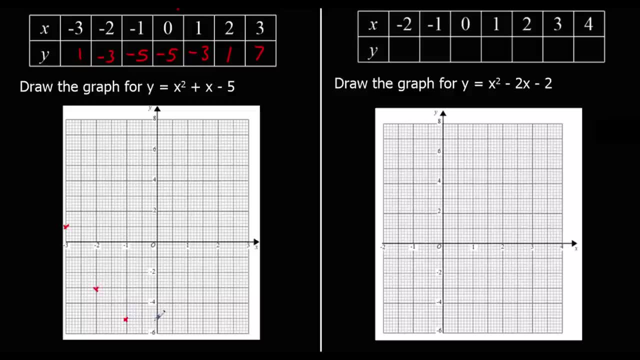 1 negative, 2 negative, 3 negative, 1 negative, 5, 0 negative, 5, 1 negative, 3, 2, 1 and 3, 7, and we're going to join these up with a curve. it's going to be a nice u shape. 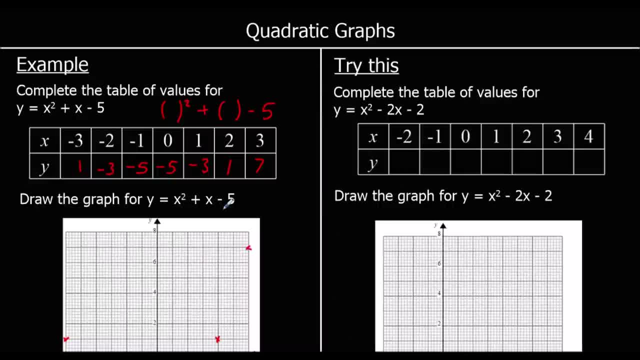 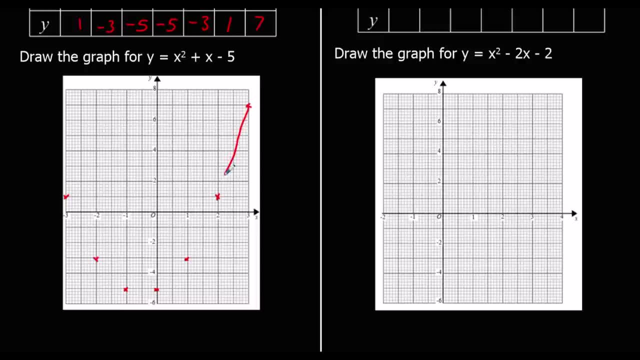 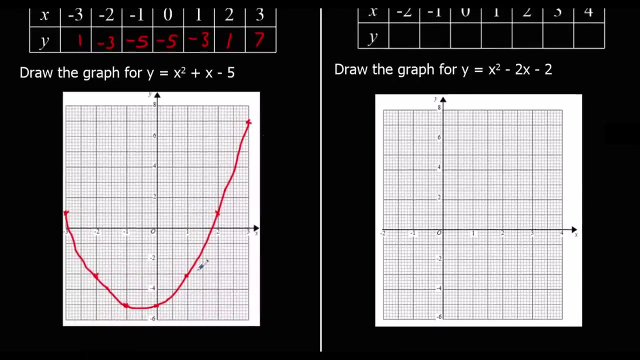 like the ones we had drawn for us, and you should get a nice symmetrical pattern as well, and you should get a nice symmetrical pattern as well. so it looks something like that. ok, so that's a nice symmetrical pattern. Okay, one for you to try. 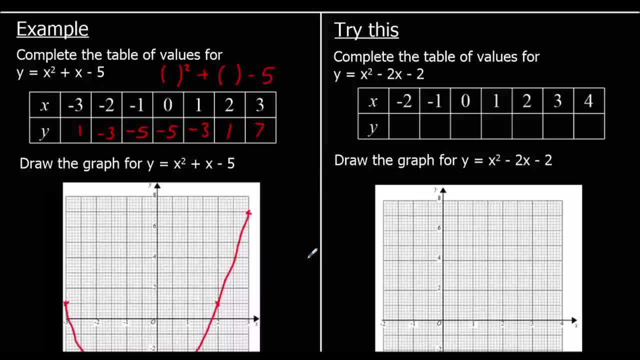 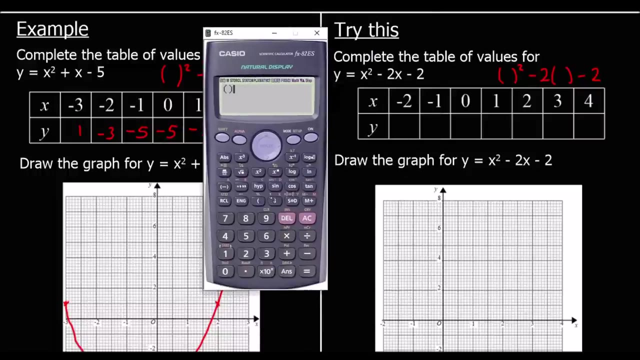 So pause the video and give this a go. So if you're going to work these out in a calculator, remember to use brackets. So replace the x's with brackets And then just substitute your x numbers into the brackets. So x squared minus 2x minus 2.. 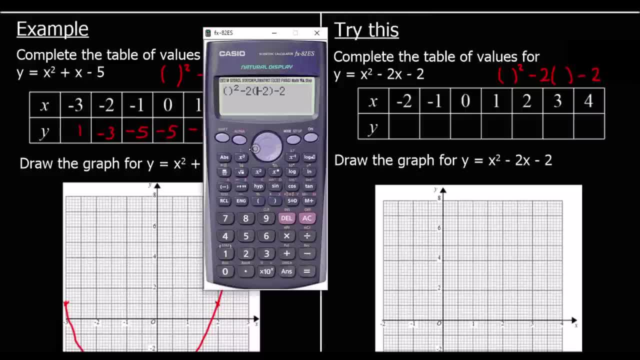 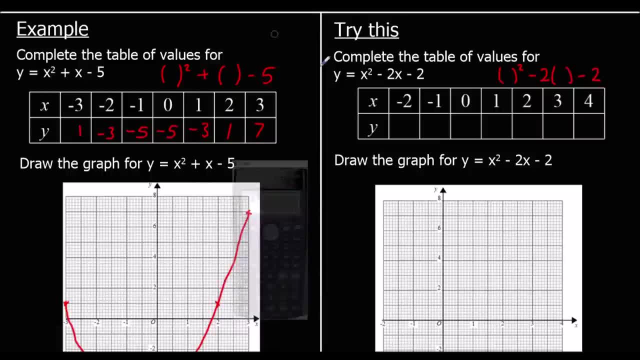 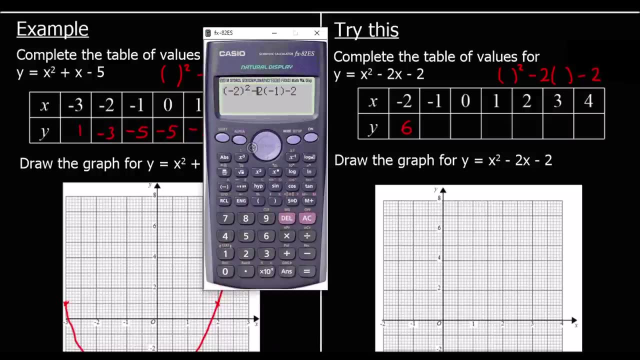 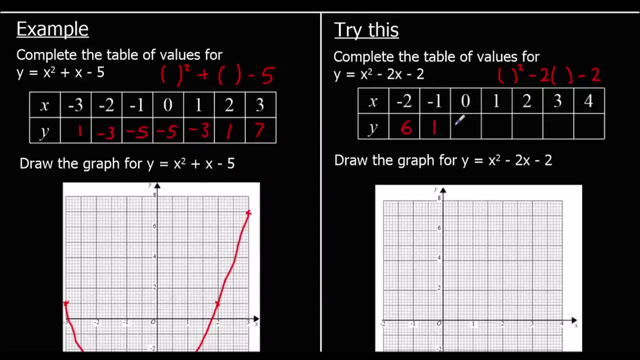 So if we start with negative 2, that's 6.. Negative 1, 1.. 0 will be negative 2, because 0 squared minus 2 zeros is 0.. Minus 2 is negative 2. And the pattern: minus 5 minus 3.. 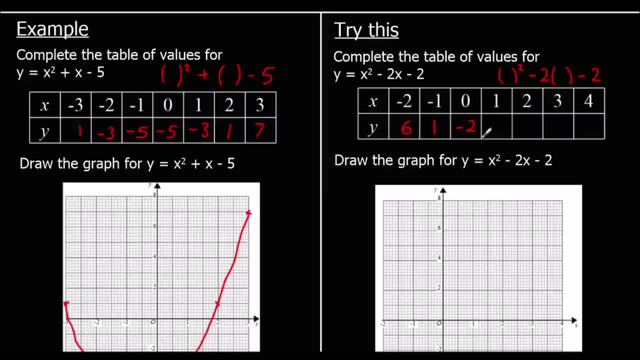 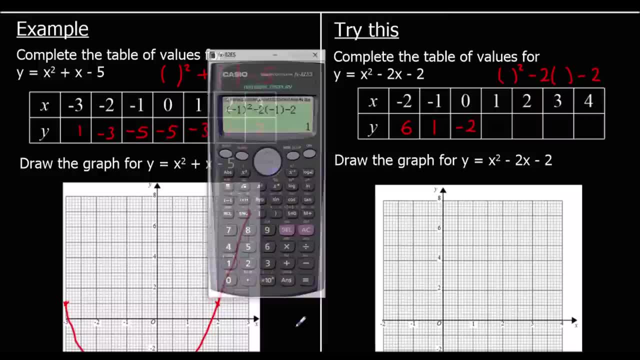 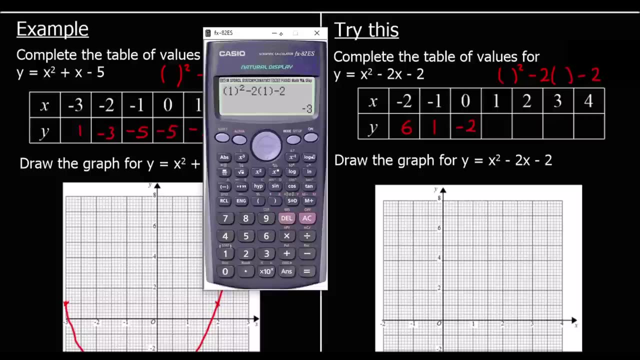 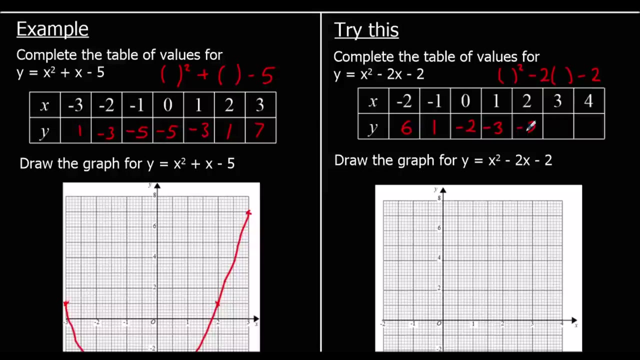 Minus 5, minus 3.. Then it'll be minus 1.. Then plus 1 plus 3 plus 5.. But we can check on the calculator: So down 1,, so down 5, down 3, down 1, up 1, up 3, up 5.. 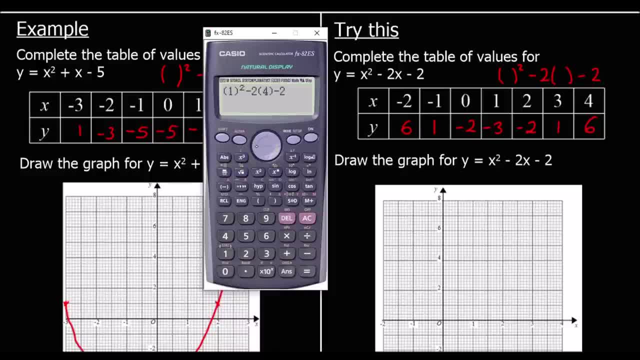 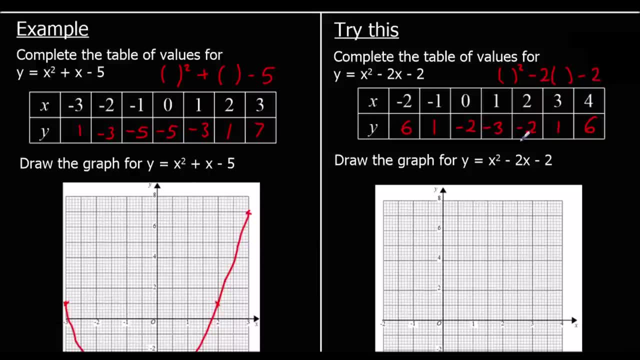 So let's just check: When x is 4, we should get 6. And we do, So we've got a nice symmetrical pattern for our quadratics. Because the graphs make a nice symmetrical pattern. Because the graphs make a nice symmetrical pattern. 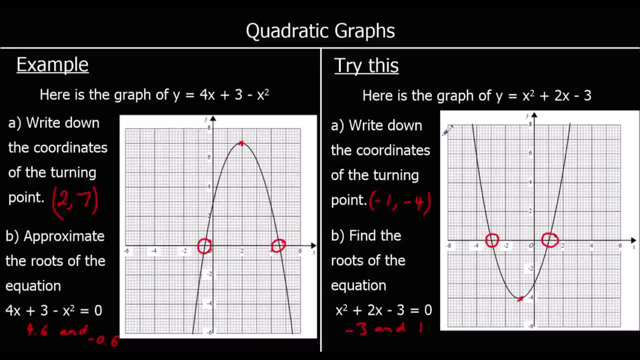 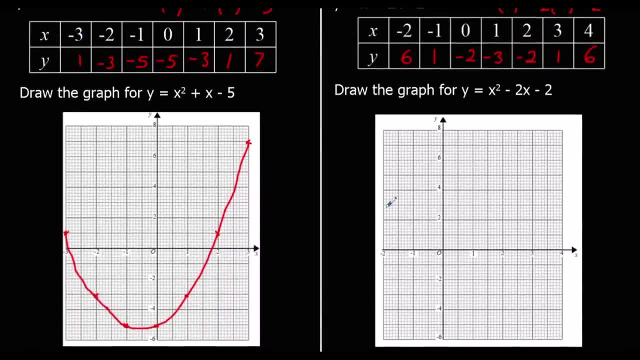 Because the graphs make a nice symmetrical pattern, Because the graphs make a nice symmetrical shape. So we get a symmetrical pattern And we're going to plot these points on. So negative 2, 6.. Negative 1, 1.. 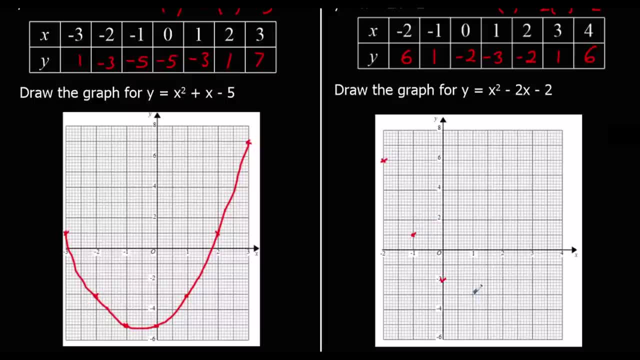 0, negative, 2. 1, negative, 3. 2, negative 2. 3,, 1.. 4,, 6.. And again, let's join them up with a nice smooth curve if we can. And there is our graph. 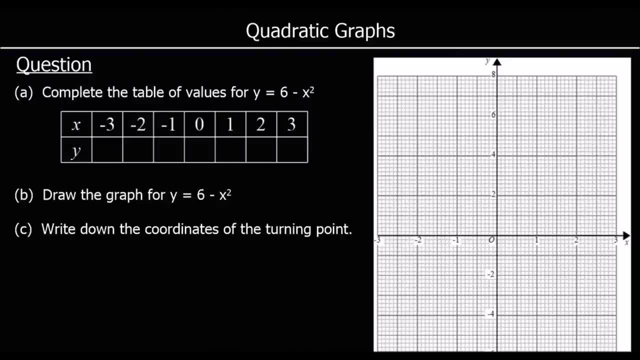 Okay, One more question to finish up. So we've got to complete the table of values, Draw the graph And then write down the values, And then write down the coordinates of the turning point as well. So we've got y equals 6 minus x squared.